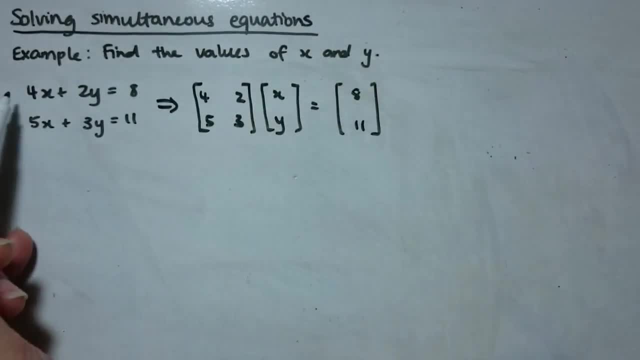 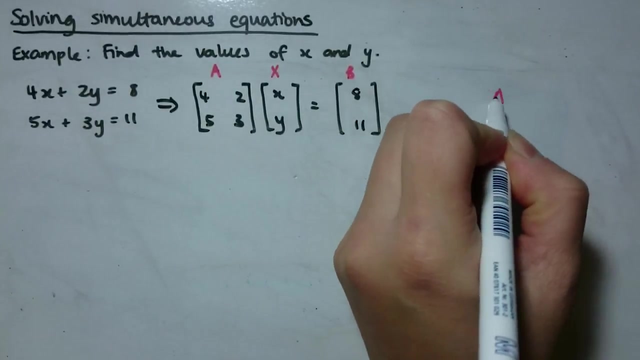 element: 4 times x for x plus 2 times y, which is this left hand side here. So that's why we set up the equations like this. Again, this is not something you have to do every time. If you name them- a, x and b, what you've actually got over here is ax equals b. You want to? 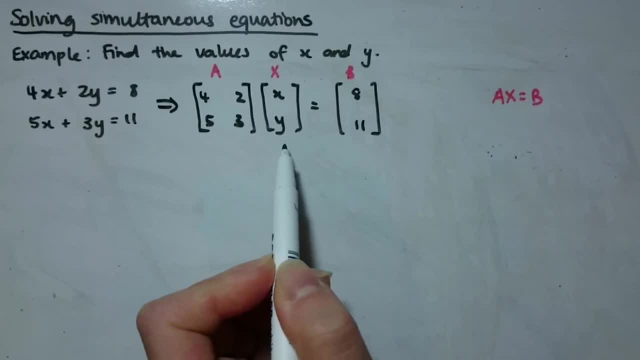 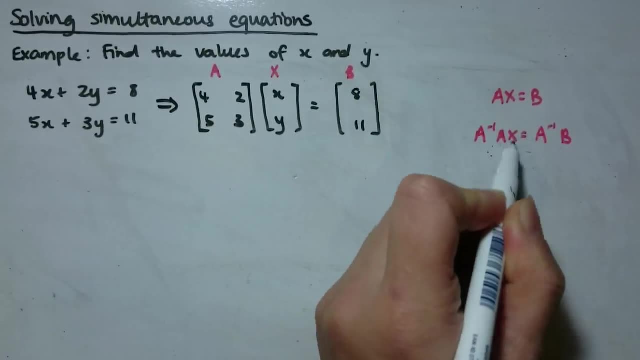 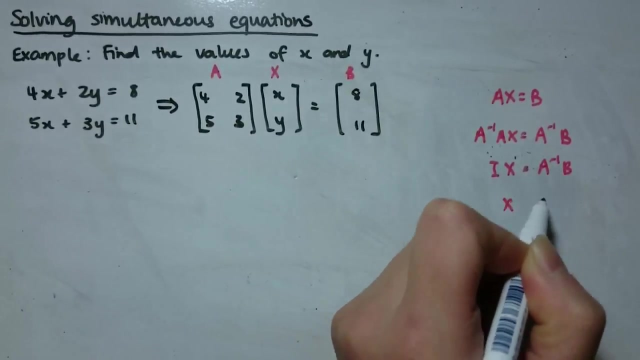 solve this equation for the matrix x so that we can work out the values of x and y. Remember, pre-multiplication by the inverse a. inverse times a is just the identity and the identity times anything is just x. So we get that. That's what we're looking for here. 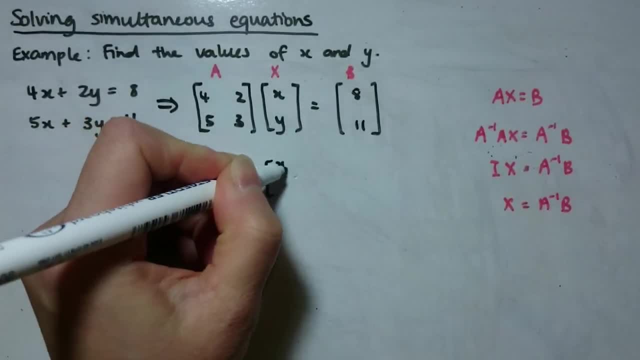 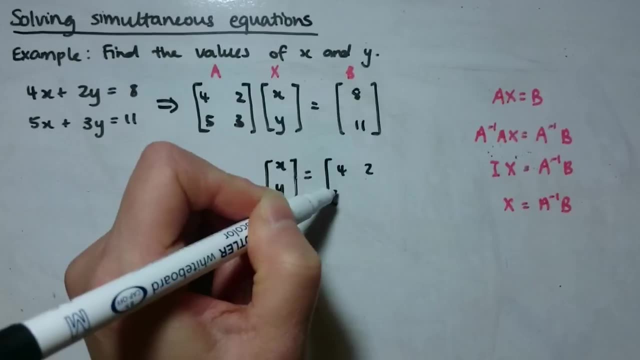 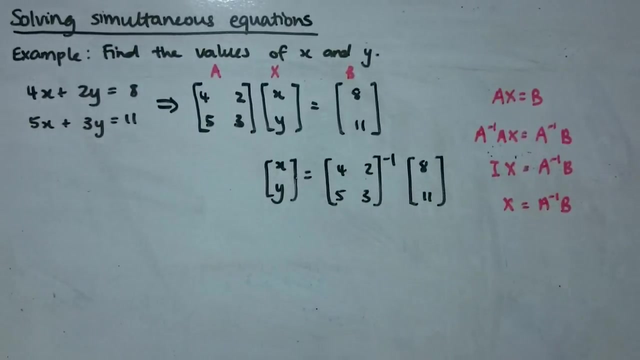 When we want to solve for this matrix x- y, what we actually want to do is we want to find the inverse of a first. So a inverse here and multiply that by the b. We're going to be able to work out what the values of x and y are. Remember to find the inverse. 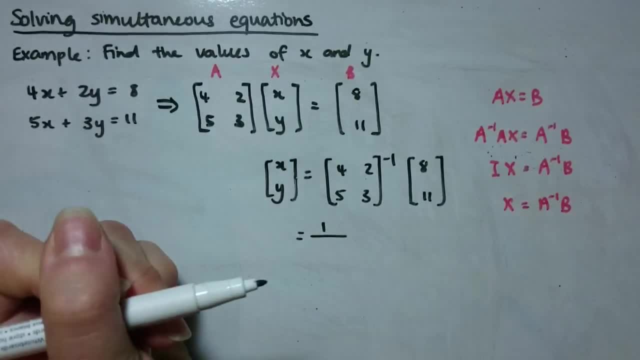 of a two by two matrix, you need to do 1 over the determinant. The determinant here is 4 times 3 is 12. Takes away 5 times and gets 0. If it's 2 by 2 matrix, you've got two again. 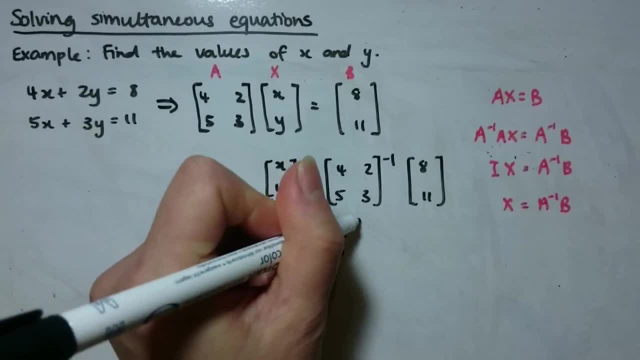 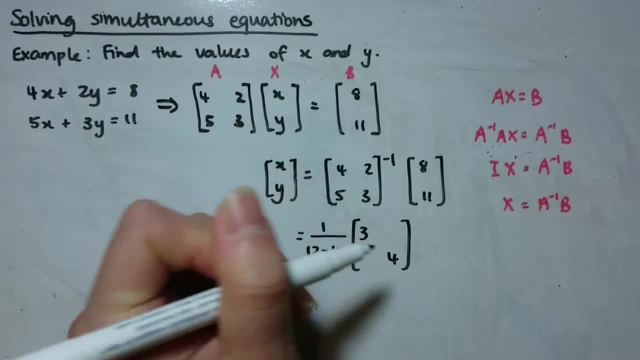 So you only conquered one line. NowVISAmakeHatscom times 2 is 10.. And then with this matrix in here we've got to do some things with the elements. So we're switching 4 and 3 on the main diagonal And we are changing the sign of the elements. 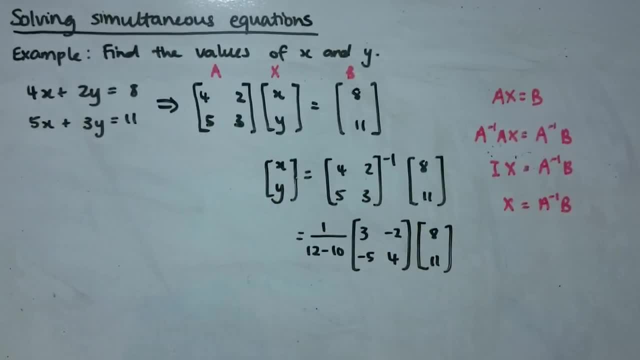 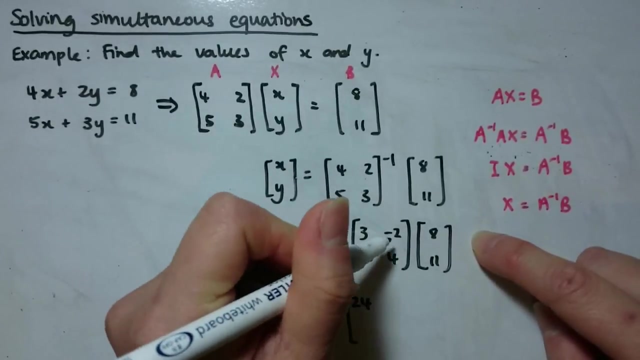 that are not on the main diagonal. Again, I'm just going to leave this as a fraction out the front and do the multiplication with integers, because that'll make it a little bit nicer. So remember matrix multiplication again, row by column. So 3 times 8, 24.. Negative: 2 times 11,. 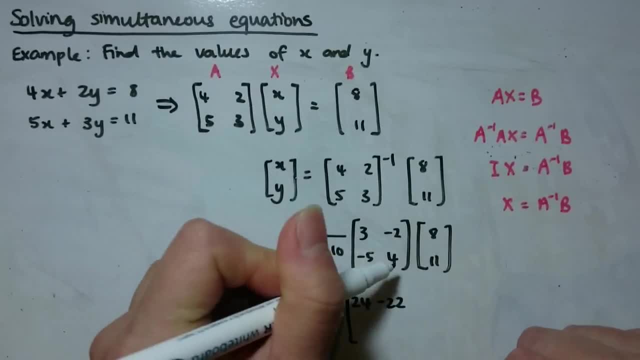 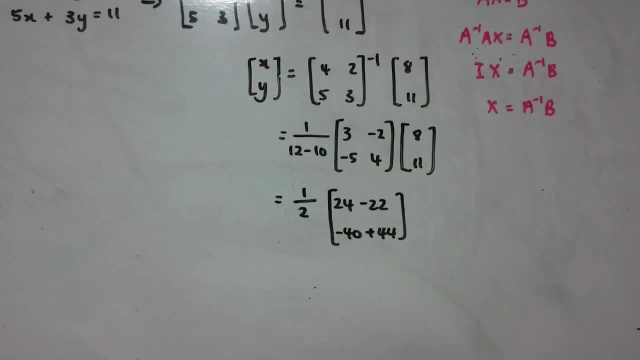 22.. Negative 22. And then the second row by column: negative 5 times 8, negative 40. And 4 times 11, 44. So just cleaning up that matrix, there we have 2 and 4, which gives us 1, 2.. The question: 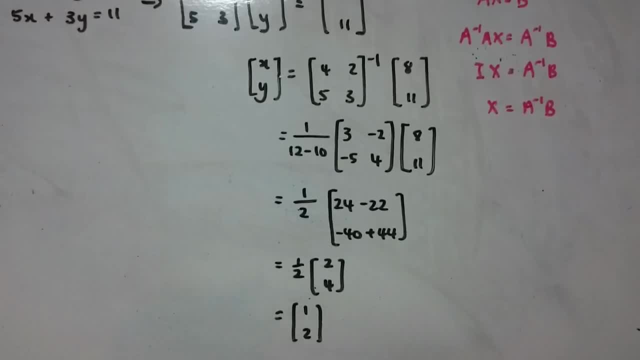 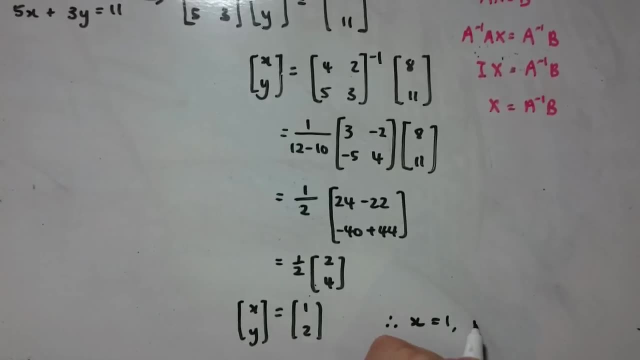 can't see it anymore, but it's. it says: solve for the values of x and y. So we actually need to state that x- this is what we have here- xy equals 1, 2.. So x is equal to 1 and y is equal to 2.. So let's just quickly check on.